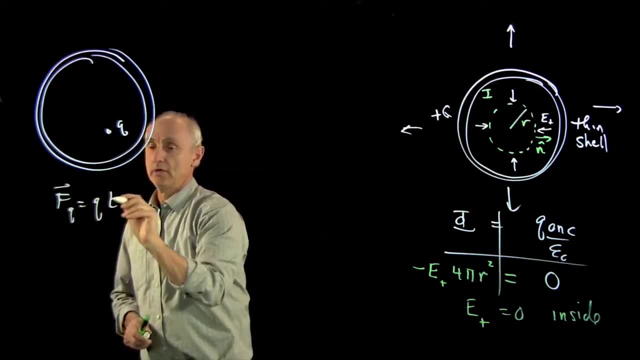 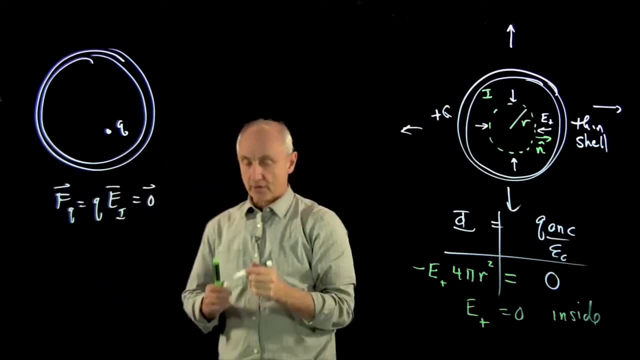 Now we've claimed, which is true, that the force on this charge is equal to the electric field times the charge, and that's 0.. But that seems very counterintuitive, because isn't this charge closer to happening? Isn't this charge closer in order to spreading the charge or the energy across the cell under any form of stream? Or are you assuming that the dynamic norm in this method takes place within the cell, or do you think it depends on the angle of 2050? I guess right now is the opposite. Now we see that the unconscious moment studied this before. Now and then ask how we view the nawet Jobs' transition of charge intoiff amper � рав drought in demand mass of 10-5i square feet. 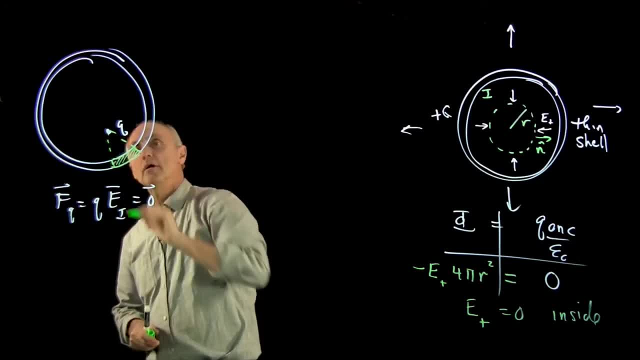 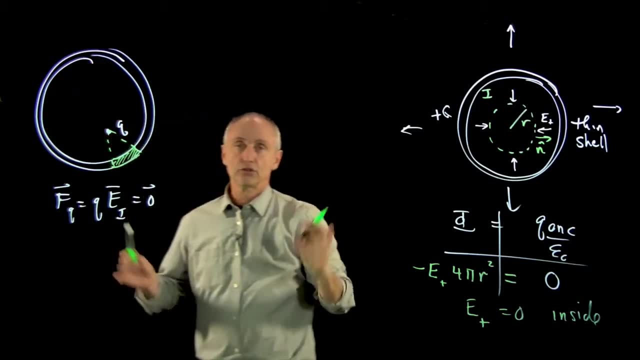 a lot of charge on the shell over here, And so that positive charge should exert a force on this. And since it's closer here, well, shouldn't that be a non-zero force? But if you think about it, let's just look at this. 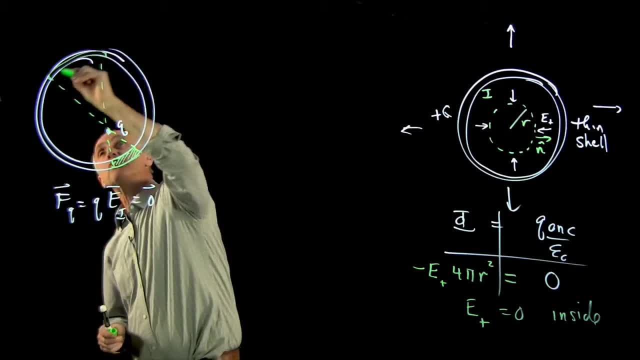 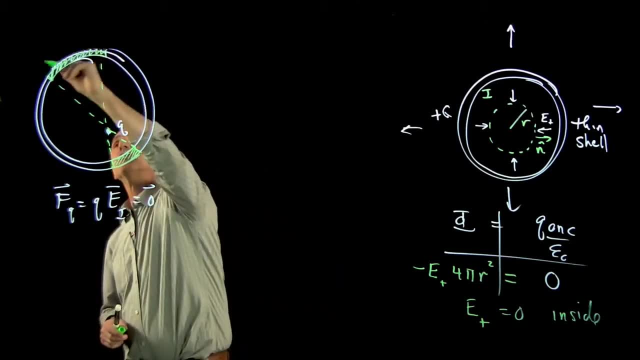 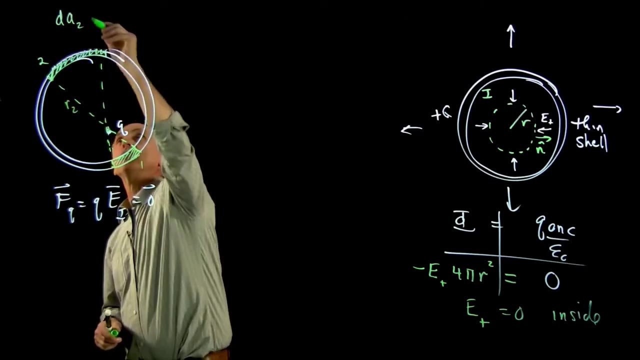 Let's extend this out and consider this part of the shell too. Now the charge is uniform, And what's interesting is they call this 2 and this 1.. The area of 2 is proportional to the distance squared. That's part of the sphere. 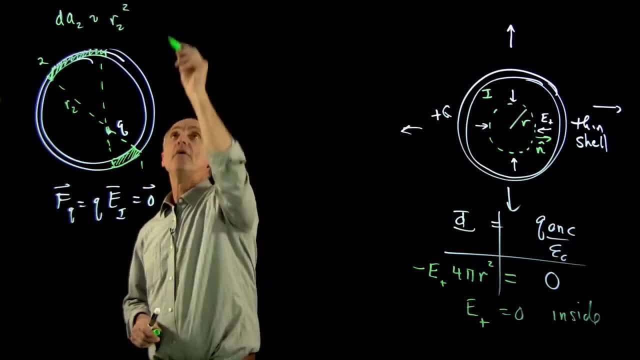 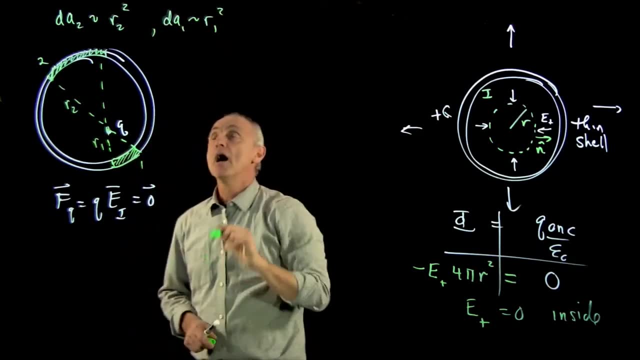 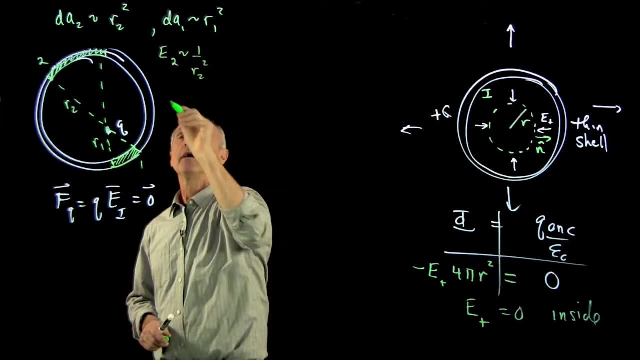 So the area on 2 is proportional to the distance squared. The area on 1 is proportional to the distance r1 squared. But the electric field of 2 goes like 1 over r2 squared And the electric field on 1 goes like 1. 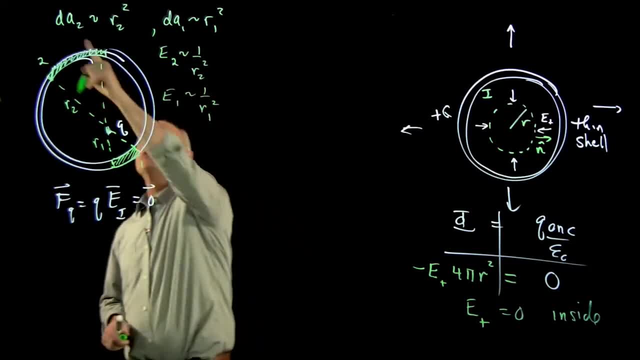 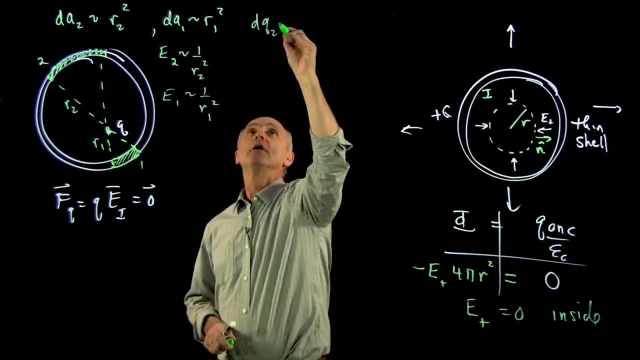 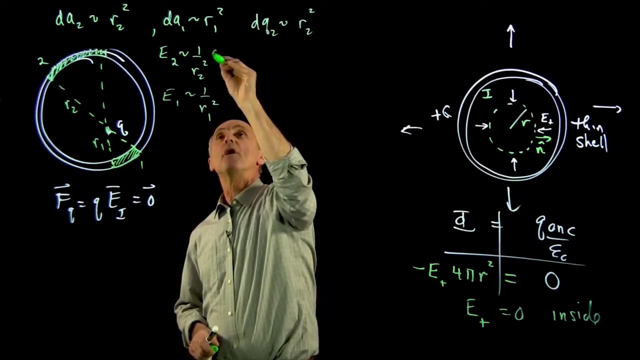 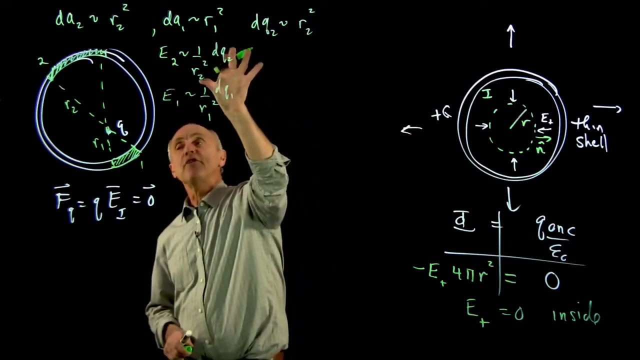 over r2 squared And the total charge is proportional to the area. So dq2 is proportional to r2 squared, But the electric field really is the product of dq2 over times dq1. And you can see that the factors of r squared. 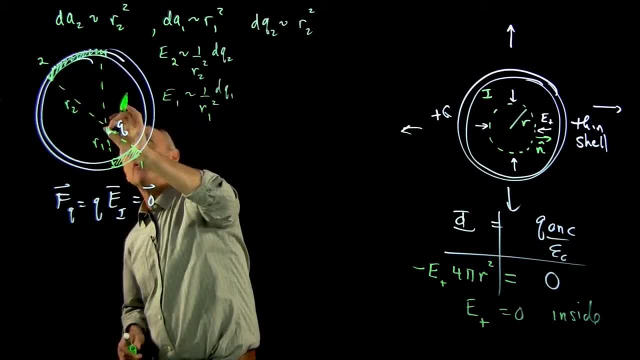 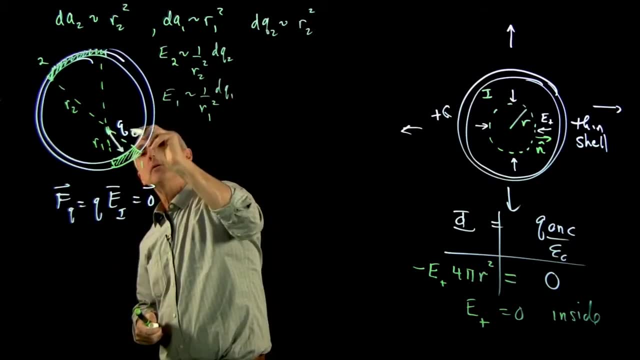 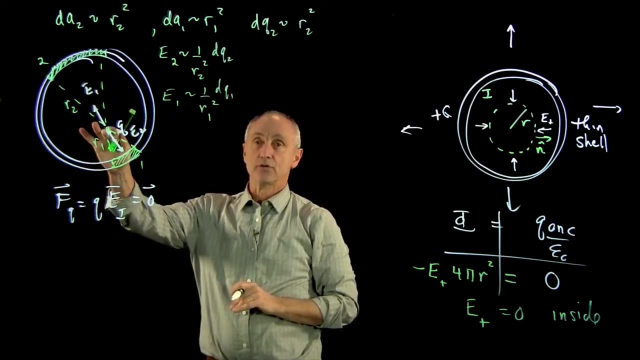 This area is bigger by r squared but the field falls off by 1 over r squared And so these two affects the effect of E2 and E1 exactly cancel, And that's why the field at some point in the center. 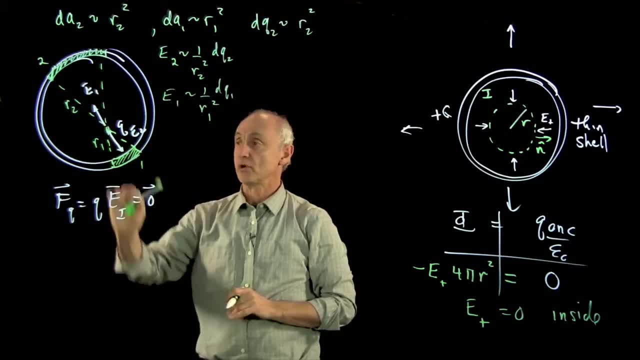 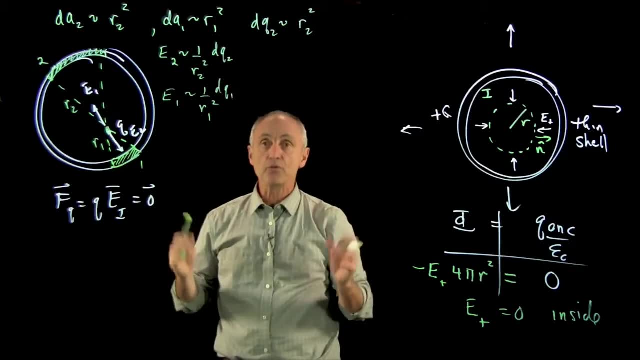 is 0 by this symmetry argument, And so the force is 0.. So even though it's closer to the side, this side still feels a force, say, in the opposite direction, And those two things will balance and you can divide up the whole shell that way. 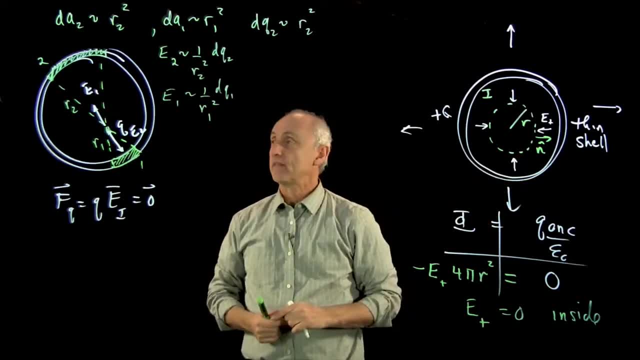 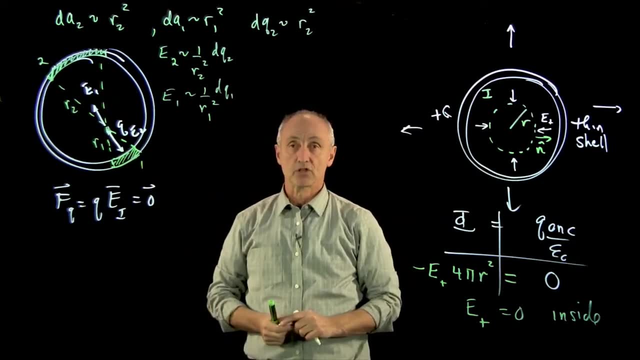 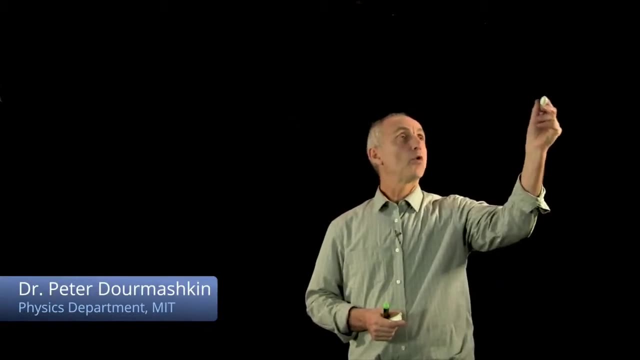 And that's why the surprising result that the electric field is zero inside the shell is proved directly by Gauss's law. The symmetry argument also shows the cancellation. Let's consider one more spherical symmetric distribution of charge. Here we have a thin shell plus Q. 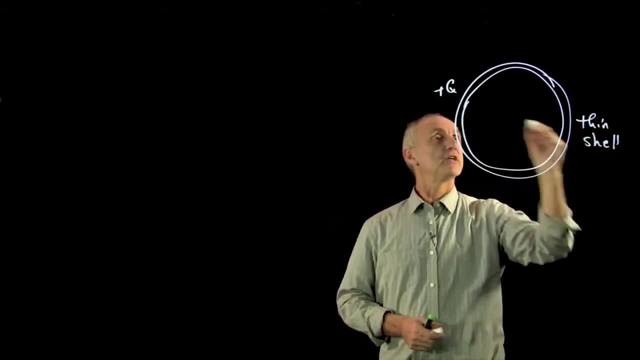 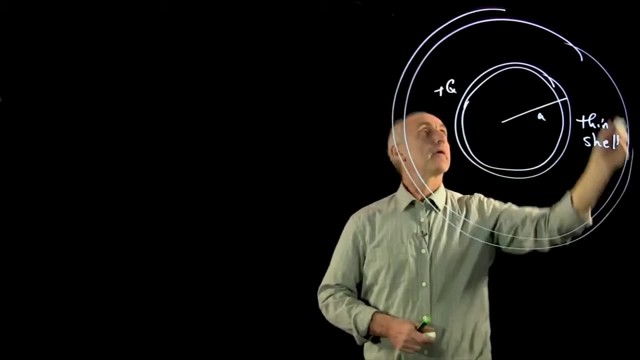 So this is a thin shell And we'll just denote the radius of the shell by A, And we're neglecting the thickness of the shell, And we're going to surround that by another thin shell of radius B, where we have a charge minus Q. 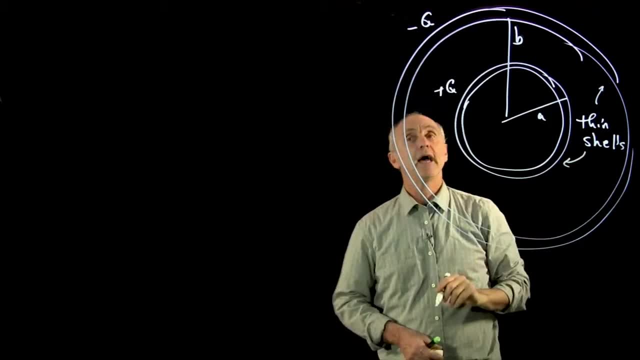 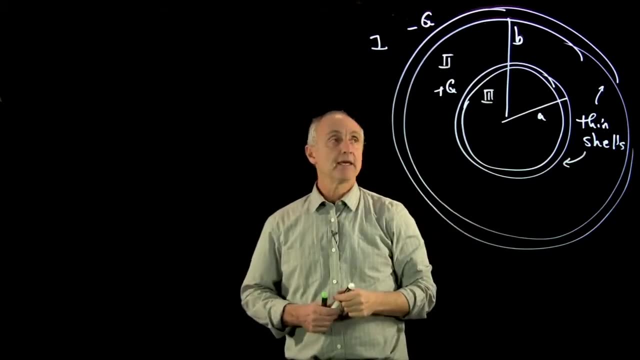 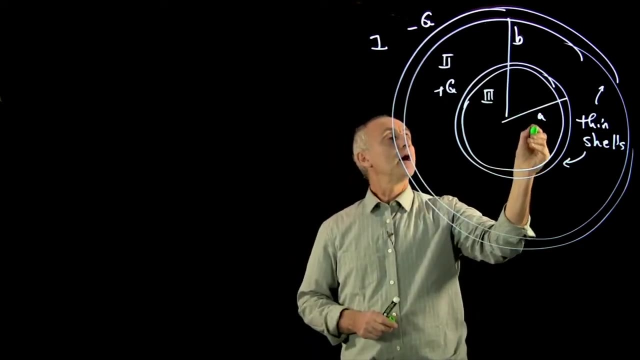 So we have two thin shells- And I'd like to find the electric field everywhere in space- And we have three regions of space. Now I want to do two of those regions very quickly. So for the region 3, I'm going to pick a region 3.. 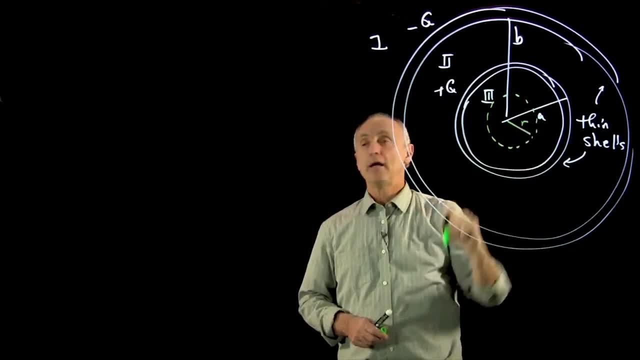 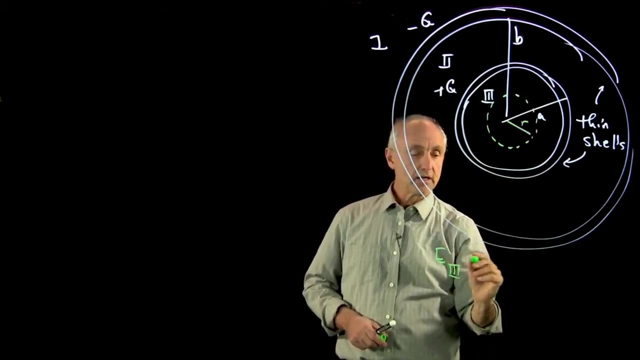 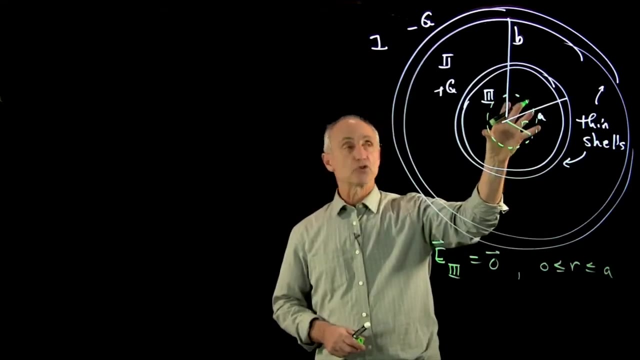 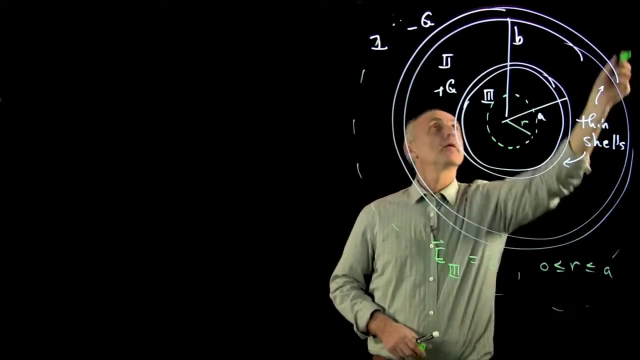 This is a Gaussian surface of radius r And in region 3, there's no charge enclosed. So the electric field inside is zero For 0, less than r, less than ay, because there's no charge enclosed in our Gaussian surface. If I do the same thing in region 1,, 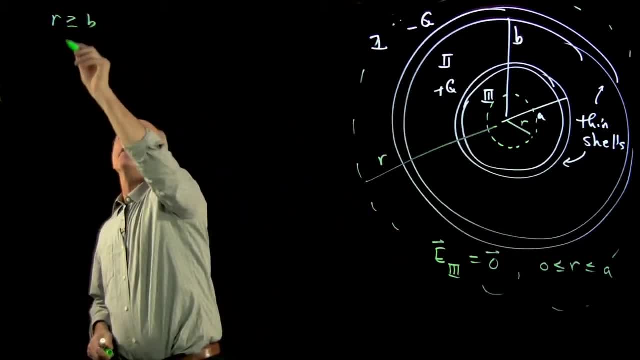 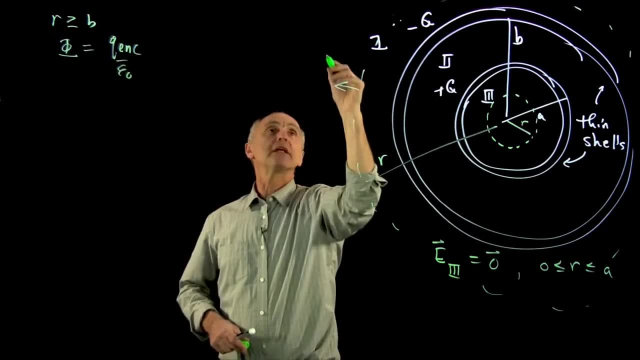 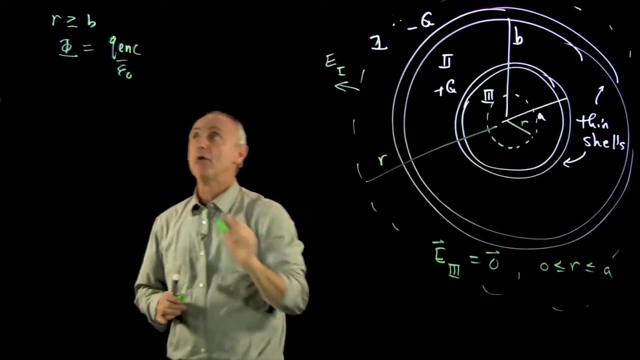 so for r bigger than b, our flux equals Q enclosed over epsilon 0.. Well, the flux is the usual. Let's just conjecture that there's an electric field. We don't know yet, We'll just conjecture. But it has to be radially outward. 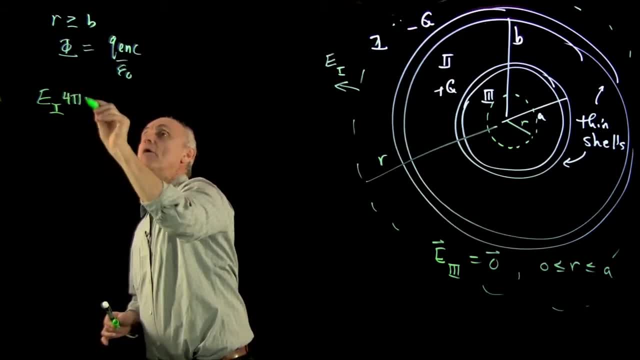 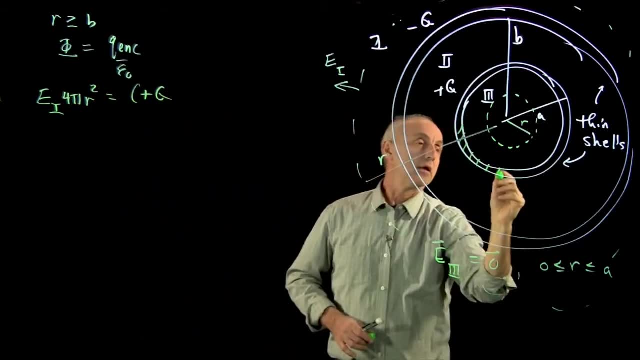 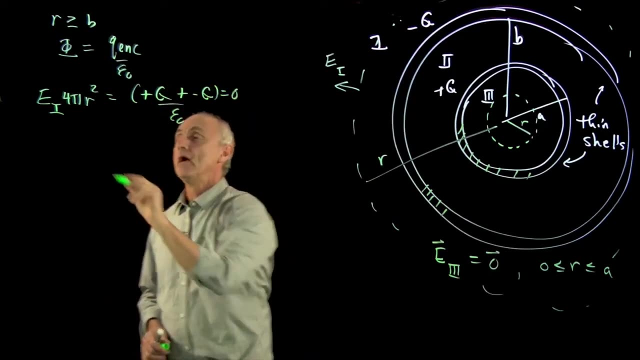 So this side would be E1 times 4 pi r squared, But the charge enclosed is plus Q, this one And minus Q the outer one, and so that's 0.. And so once again, we conclude that the electric field. 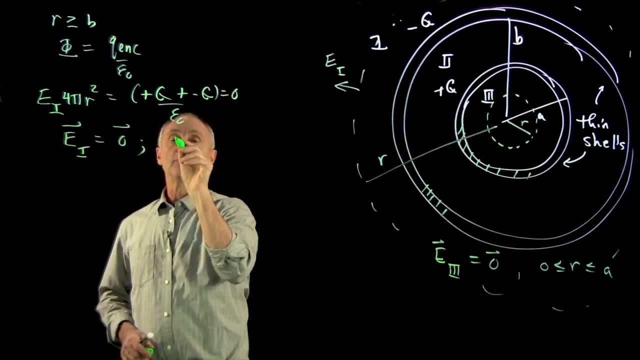 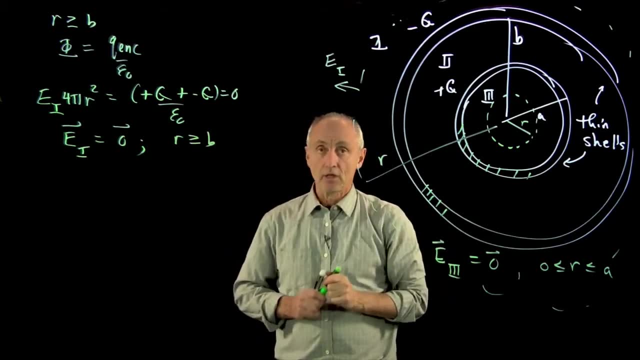 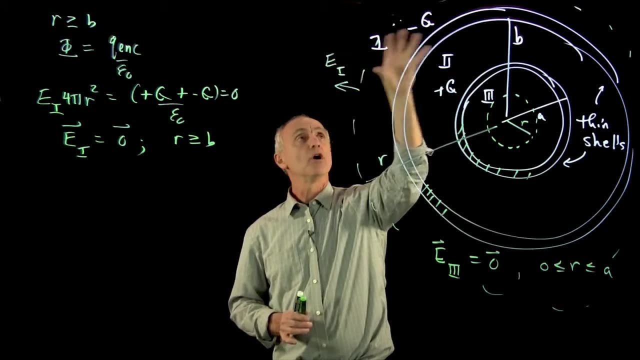 outside the shells is 0.. And this is r bigger than b. And now, if you wanted, you could think about this as a superposition problem, where you just calculated the field of a negative shell and added it to the field of a positive shell outwards.